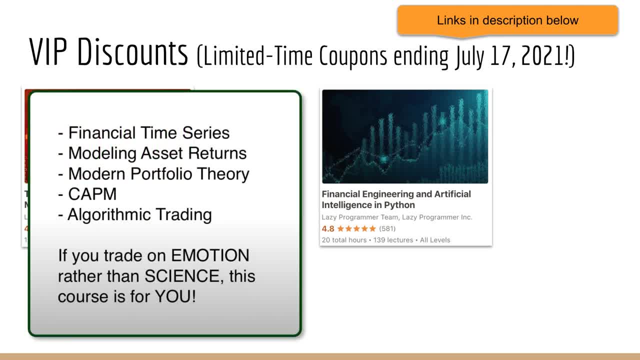 time-series. In my financial engineering course, we not only cover financial time-series, but also how to build an optimal portfolio and how to trade using algorithmic rules. If you tend to trade in the stock market using your emotions rather than science, this course 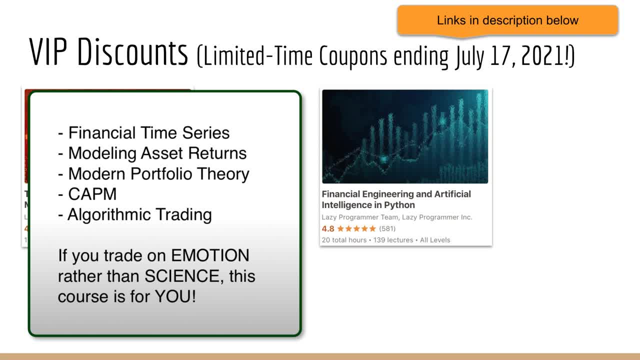 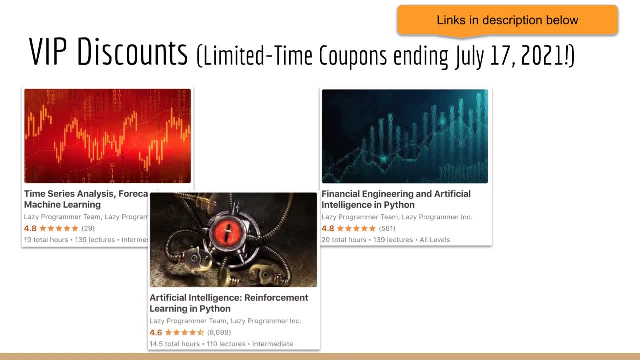 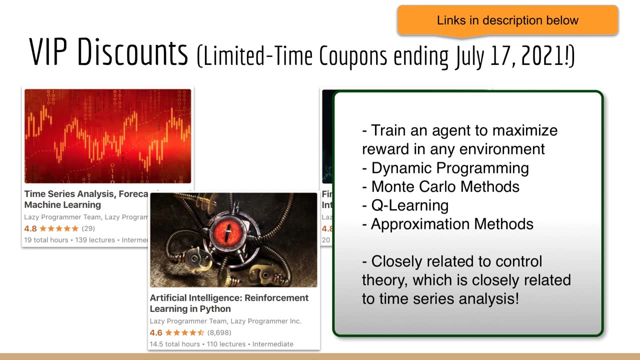 is for you Now. it turns out that there is a whole field of study devoted to learning these algorithmic rules such that you can maximize your reward. This is the field of reinforcement learning. Reinforcement learning also happens to be very closely connected to control theory. 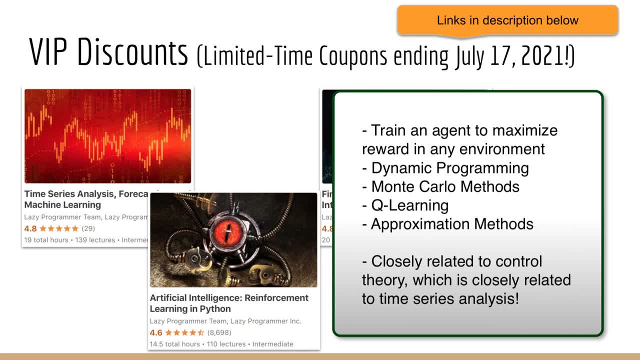 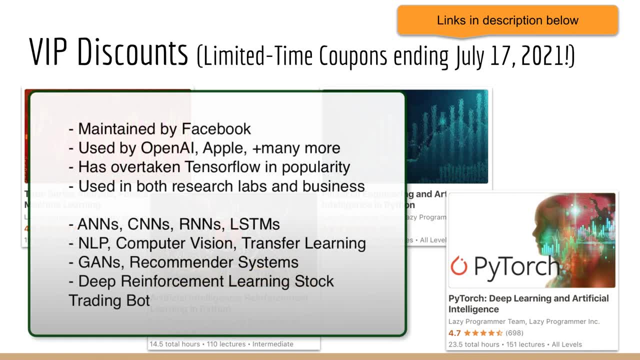 which, as you'll see, is sort of like a cousin to time-series analysis. The final VIP course I want to mention is my PyTorch course. Now, I probably don't have to tell you this, but deep learning is one of the most important topics in data science. 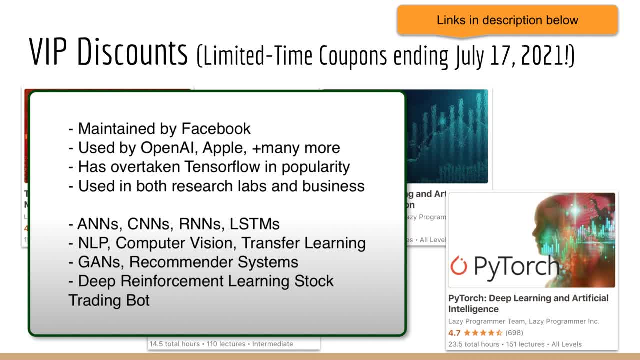 nowadays, The preferred library used by most leading companies and research labs is PyTorch. TensorFlow used to be cool, but its popularity has decreased over the years. It's been a long time since I've used it and it's been a long time since I've used it, but it's. 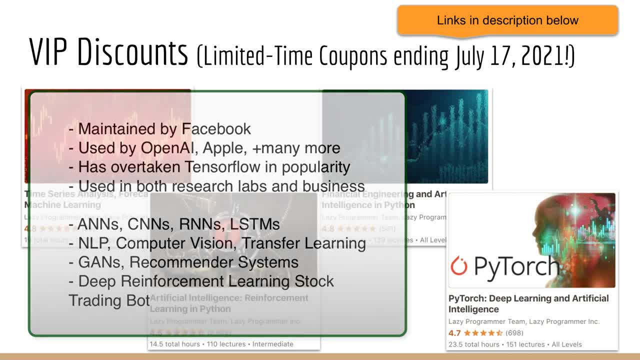 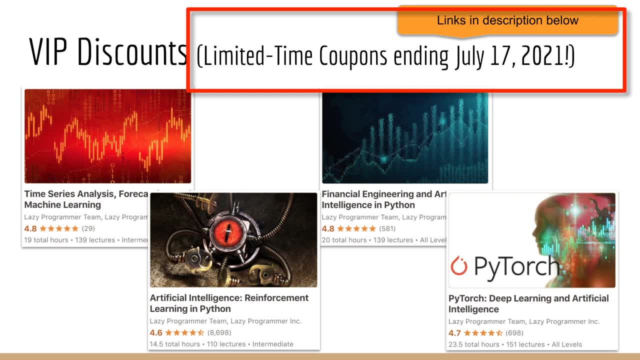 been a long time since I've used it. Okay, so again, these coupons expire in less than one week. You can find the VIP links in the description below. Now, importantly, if you watch this video too late, you may still have a chance to get the VIP coupons. So check the links in the description to see. 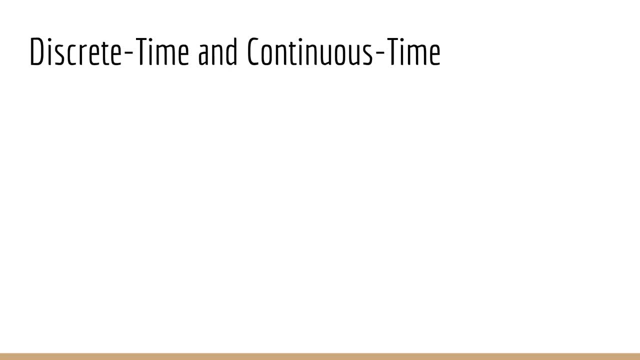 if there are any updates. Okay so let's start with one surprising fact, which is that states-based models can be applied in both discrete-time and continuous-time systems. Okay so let's start with one surprising fact, which is that states-based models can. 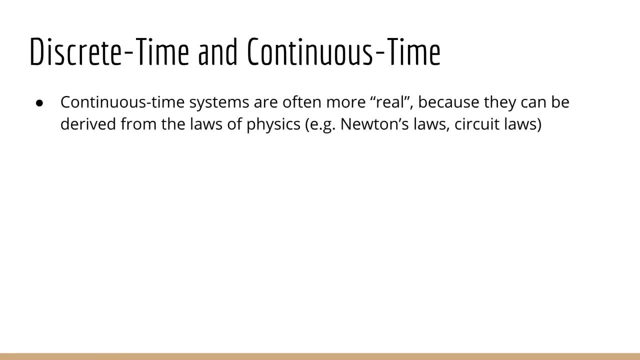 be applied in both discrete-time and continuous-time systems. Continuous-time systems are often more realistic because they correspond to the laws of physics, but eventually you have to program these systems into a computer which requires a discrete-time representation. The most common type of states-based model is the linear states-based model, which 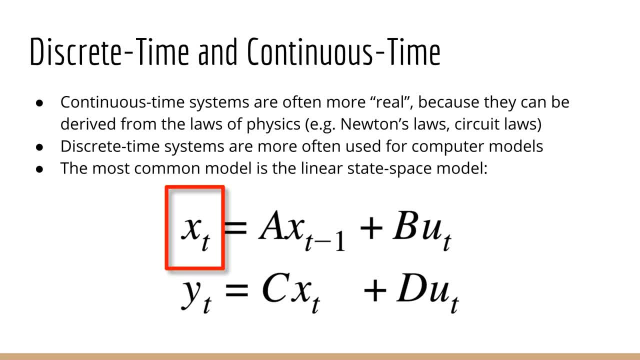 looks like this. This discrete-time version says that the state vector at time t depends on the previous state vector at time, t-1, and some control input vector u. The relationship between these vectors is controlled by the first state vector at time, matrices A and B. The output vector y of t depends on the state vector and the control input through. 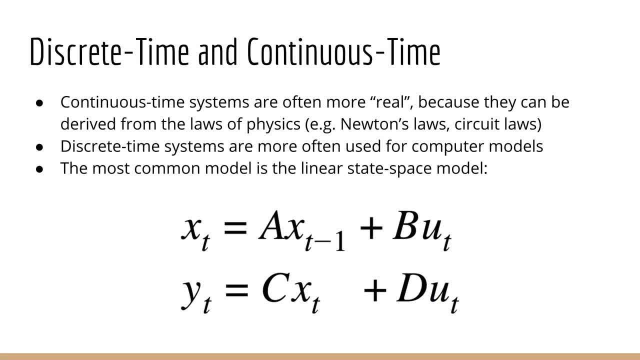 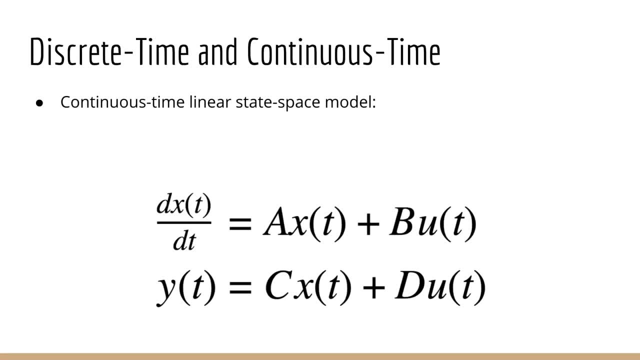 the matrices C and D. Now don't worry if this seems a bit abstract, since we'll do an example very shortly. So here's a linear state-space model in continuous time. Basically it has the same format as the discrete-time version, except that on the left side we have a time derivative instead. 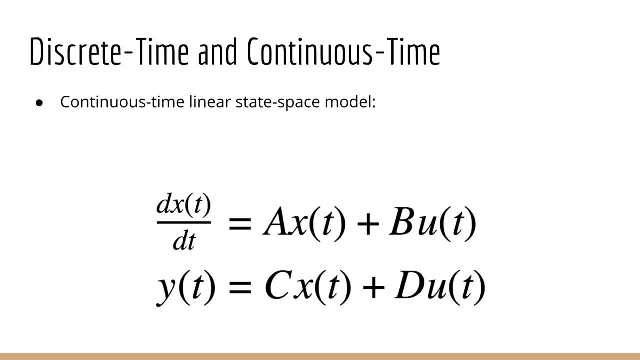 of just the next time step And again. continuous time systems are useful because they can represent real physical laws of nature, So any analysis we do on these systems is based on real physics. This is opposed to discrete-time systems, which are more useful for building computer programs. 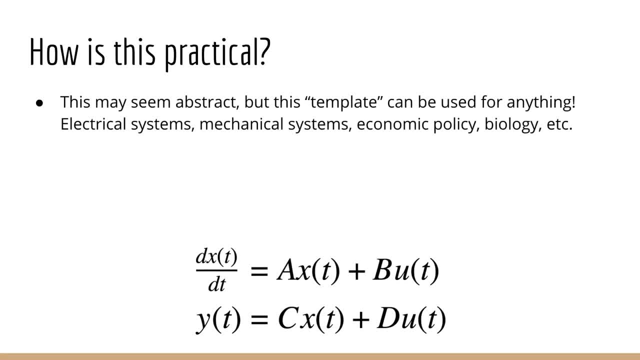 Okay. so, as mentioned earlier, although these equations may seem a bit abstract, they are also very general. What we discuss in this lecture can really be applied to any field, whether that's electrical systems, mechanical systems, economic policy and biological systems. 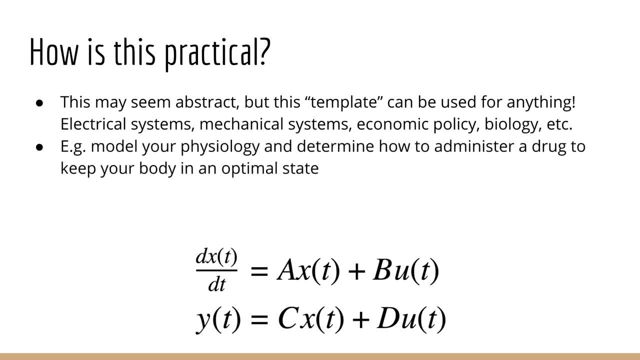 So, for example, you can model your physiology and determine how to administer a drug to keep your body in an optimal state. For this video we'll be doing a simple example which only requires a bit of high school physics. So hopefully it makes sense and you recognize. 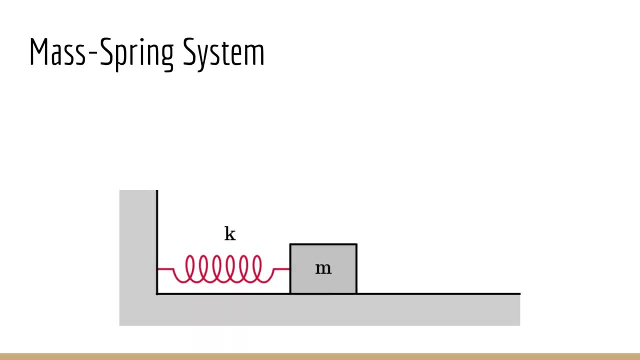 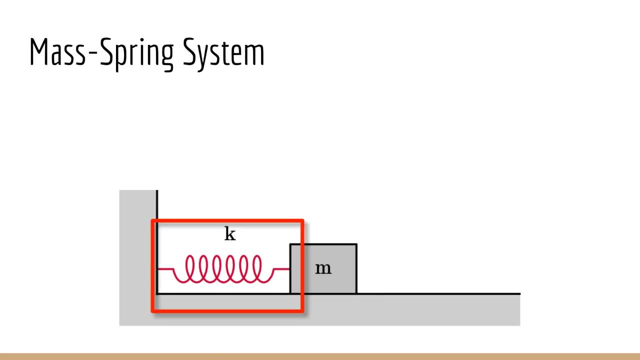 The mass in the spring is the mass in the spring. So let's suppose we have a mass attached to a spring which is attached to a wall on the other end. Now, as you recall, our goal in such a system is to determine all of the forces that can act on each mass. In this case, we only have one mass. 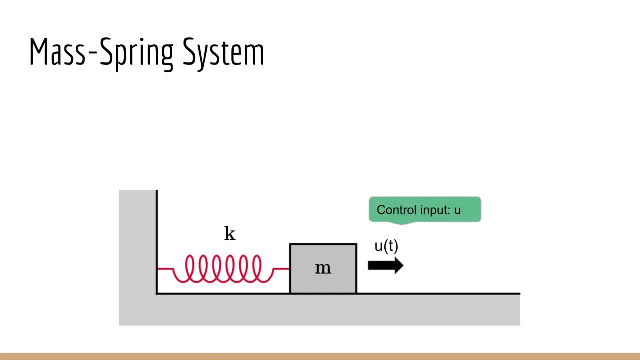 So one force on this mass is the input force, U, which is the force that we get to apply. So you can imagine this like being the output of your computer program that gets to control how much force is applied to the mass. Now this is not the only force applied to the mass. 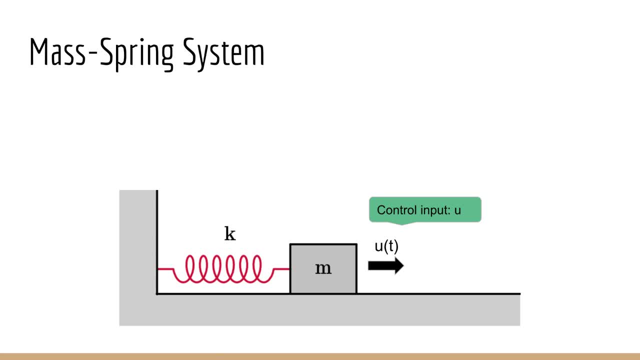 The spring also applies a force whenever the spring is not in a neutral position. So let's create a variable, x, which represents how far away the mass is from its neutral position. Thus x equals zero, represents no tension on the spring. We'll assume that the positive direction is left to right, so that when the mass 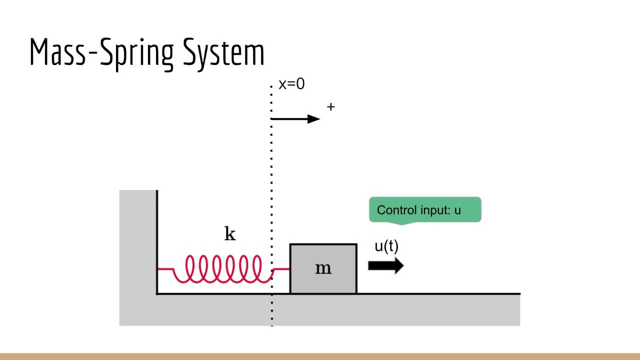 is to the right of this neutral position, then x is positive. In this case, the force from the spring is minus kx, where k is what we call the spring constant. This force has a minus sign because when x is positive, the spring pulls the mass to the left. Alternatively, we can just: 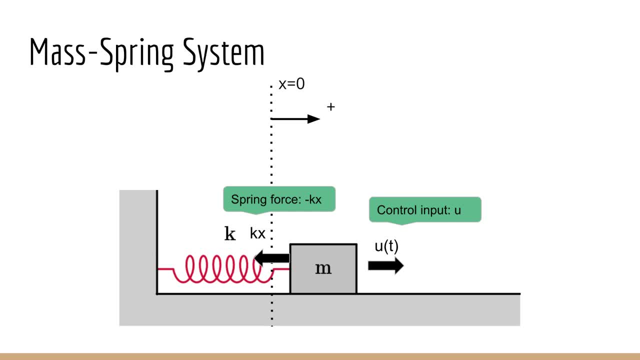 write kx with an arrow going to the left. Now there is one more force we're going to consider, which is friction. So let's assume that the mass sits on a table and this friction, or damping force, is proportional to the velocity. We'll call this damping coefficient. 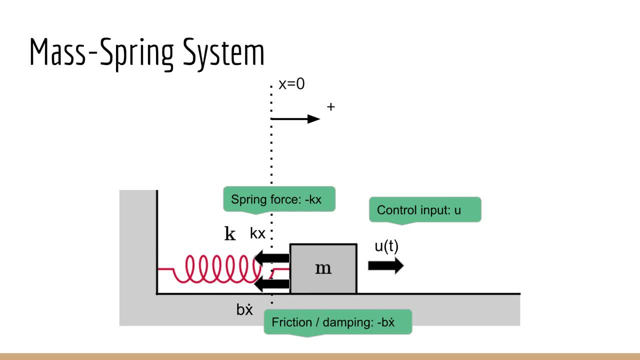 b. So the force due to friction is minus b times the velocity, or b times x dot. This has a negative sign because, again, if the mass is moving in the plus direction, this force will be in the minus direction. Also, recall that we use a dot as another way of writing the time derivative. 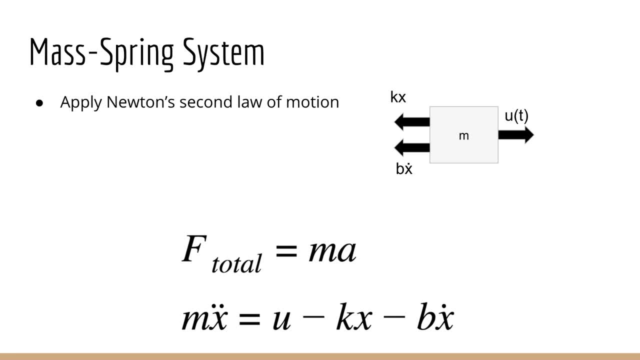 Okay, so the next step is to recall Newton's second law of motion. Basically, the force on an object is equal to its mass times its acceleration. So on the left side we have m times x, double dot Again, since the dot represents the time. 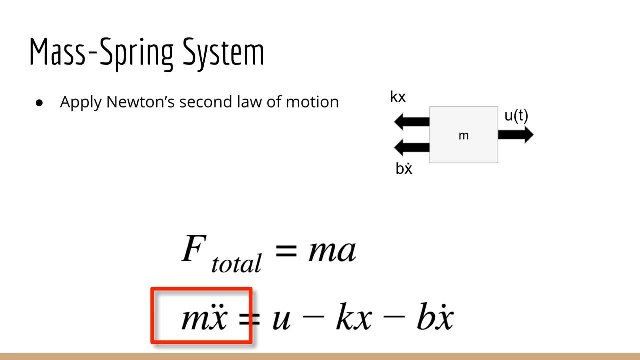 derivative x double dot represents acceleration. On the right side we have the sum of all the forces on the mass, So that's u minus kx minus bx dot. Okay, so this is an equation which represents our system. The next step is to consider how to convert this into state-space form. 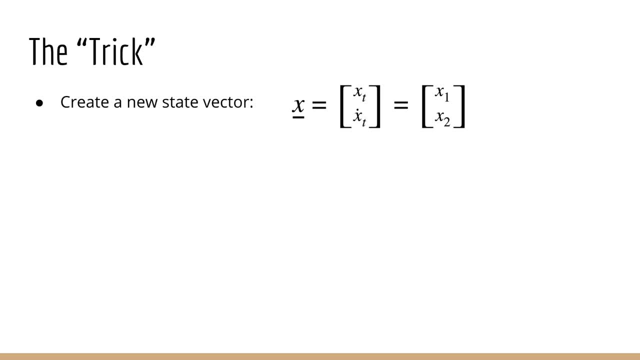 So the trick in these kinds of problems is how we define the state. In this case we're going to define a new vector containing x and x dot. So this might be a bit confusing, since I've used x for multiple things. so for the purpose of this derivation only, I'm going to use an underscore to denote the x vector. 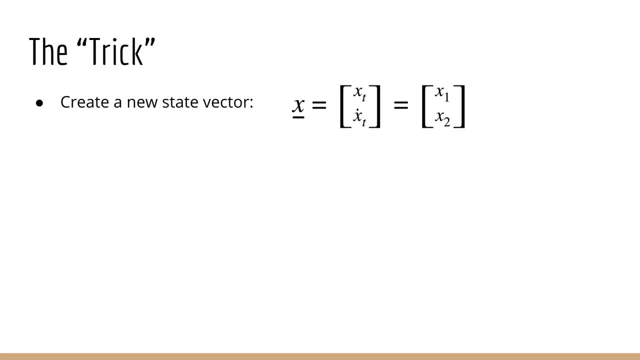 which is the state. It contains x and x dot. For convenience, we can also think of these as x1 and x2, simply the components of the state. Now, one thing we can see right away is that x2 is equal to x1 dot. The next thing to do is to express our original system. 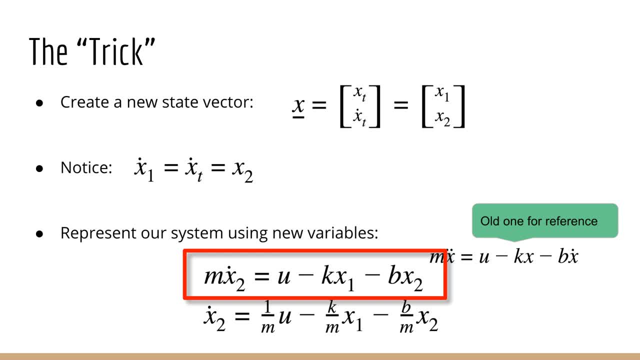 in terms of x1 and x2.. When we do that, we get m times x2 dot equals u minus kx1 minus bx2.. We can also simplify this so that we only have x2 dot on the left side. Basically, 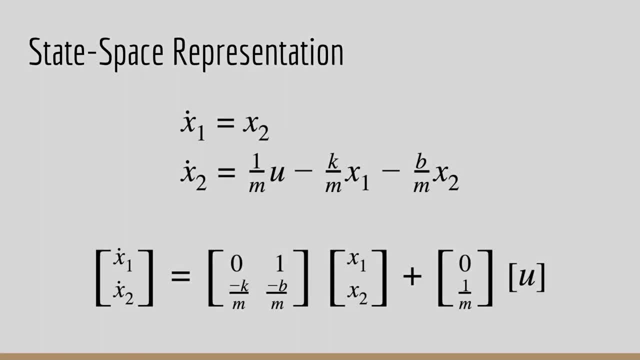 we just divide everything by m. Now, as you recall, with a state-space model, what we would like to have is the derivatives on the left and the regular variables on the right. So let's see what happens if we try to put these equations into that format. Of course, it should be clear that 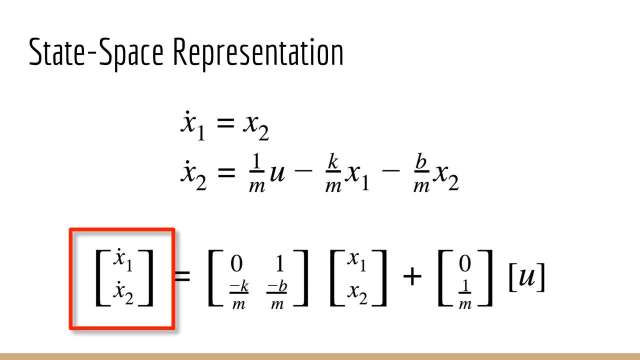 this is a matrix equation. On the left side we have x1 dot and x2 dot, which is the derivative of our state vector. On the right side, we have some matrix A multiplied by our state vector, plus some matrix B multiplied by our input u. 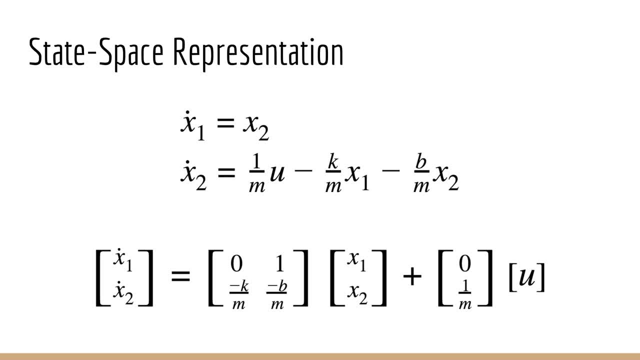 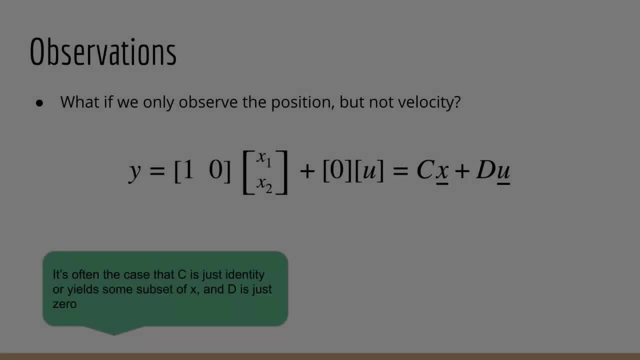 You can think of u as a one-by-one matrix. So, as you can see, both matrices A and B are determined by actual physical quantities. Now, in the real world, it's often the case that not every state variable can be observed. 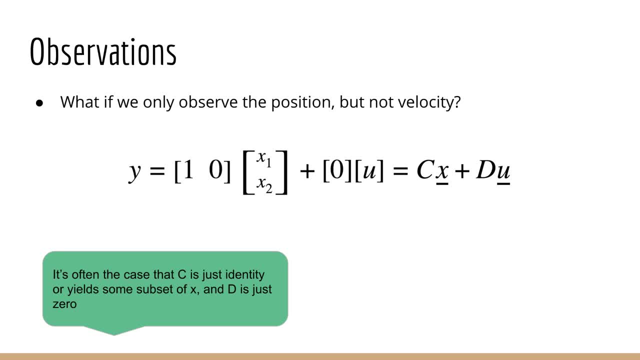 So, for example, we might know the position but not the velocity. In this case we let the variable y represent our observation, which is just the matrix C times the state vector x, plus another matrix D times the input u. Clearly, this is a pretty trivial addition to what we had before. 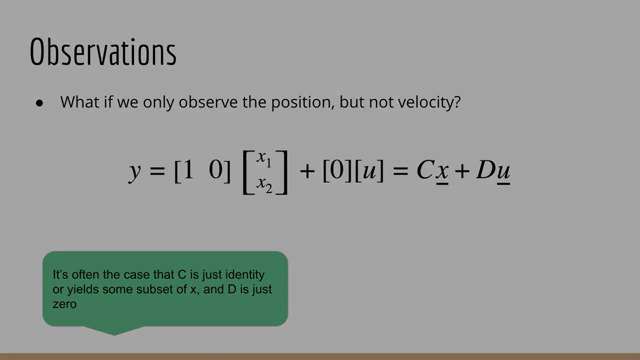 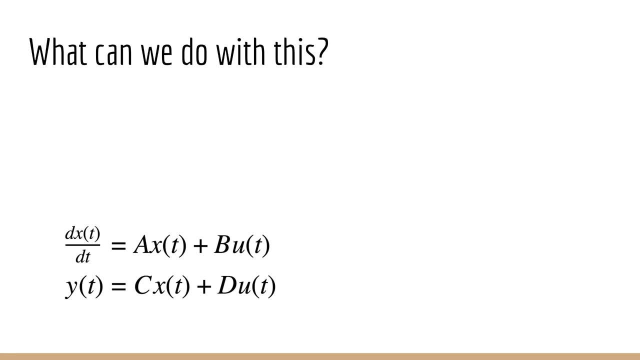 but we now have a full linear state-space representation. So this state-space representation looks pretty simple, but why do we actually care about this? Well, the fact is, there is a lot we can do with this Now. it requires some linear algebra. 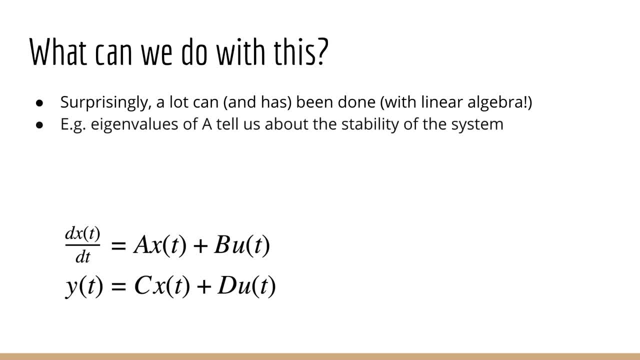 but the potential is there. For example, by looking at the eigenvalues of A, we can determine whether is stable. The most important point is that with this framework we can build programs to control these systems. So not only can we forecast the next state of the system, given where it is. 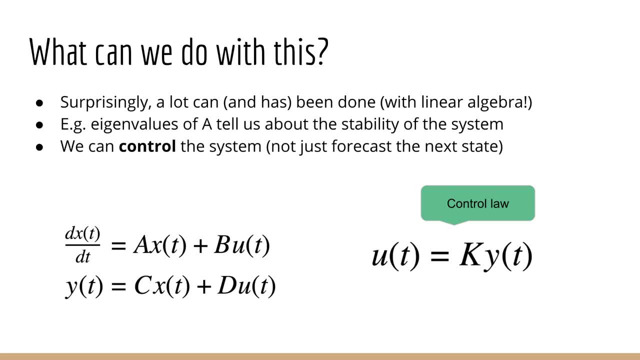 now we can actually decide where we want it to go. What we would like to do is find some matrix K such that, if we set the input U to be K times the observation Y, we will control the system in some desired way. This makes sense, since what we want to do, which is U, should be computed from. 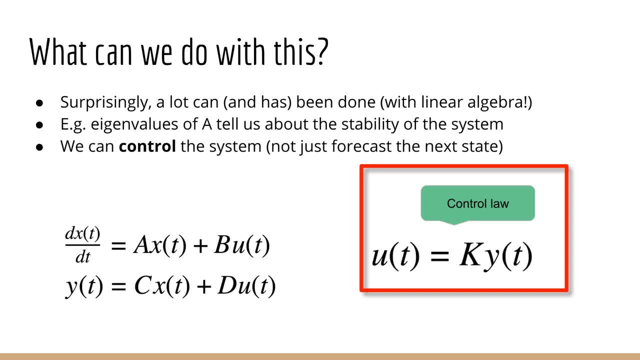 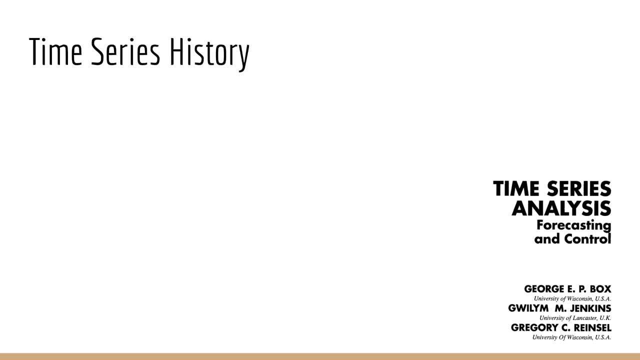 what we observe, which is Y. Of course, the challenge is: how do we actually find K? Now, one interesting fact is that one of the most popular time series models called ARIMA came from a book by Box and Jenkins. This book is really how ARIMA became as popular as it is today.